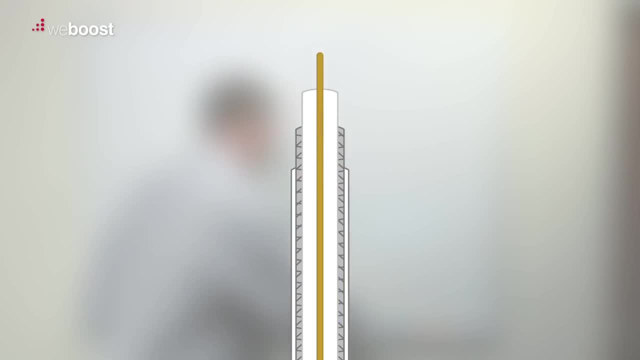 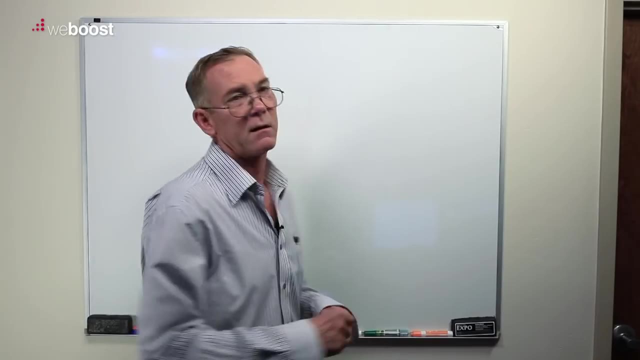 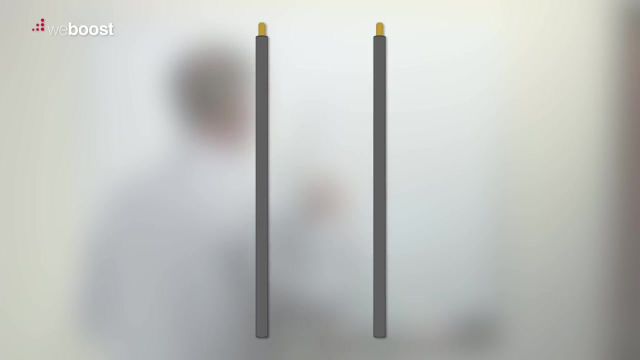 out How we get an antenna to work and actually radiate power is to change that. So to change that, we want to transmit that power out into the air. So once again you have two pieces of wire and you have current flow in this direction and current flow in that direction. A simple. 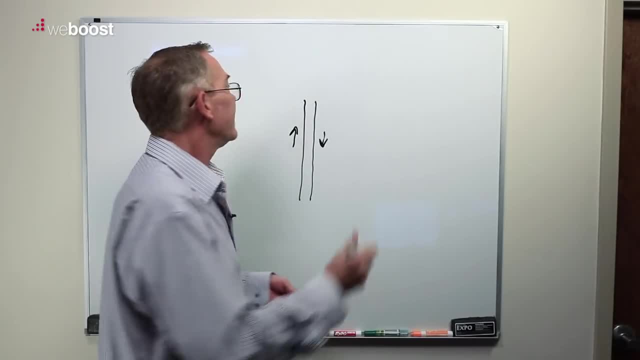 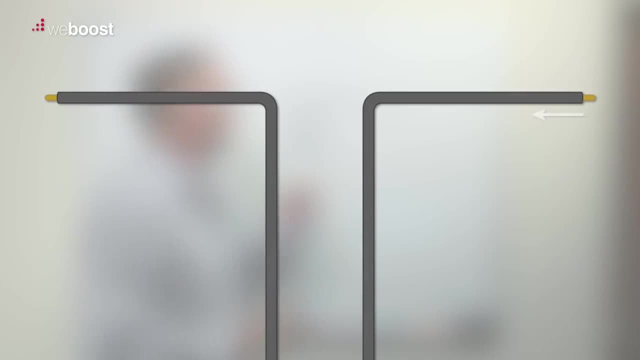 dipole antenna, like you put on your FM stereo at home, is just when you take this wire and split it off over to this direction and split it off over to this direction, And now I still have current flow in this direction and I still have current flow in this direction. 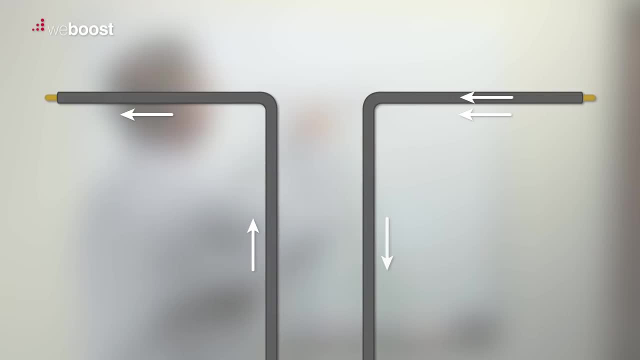 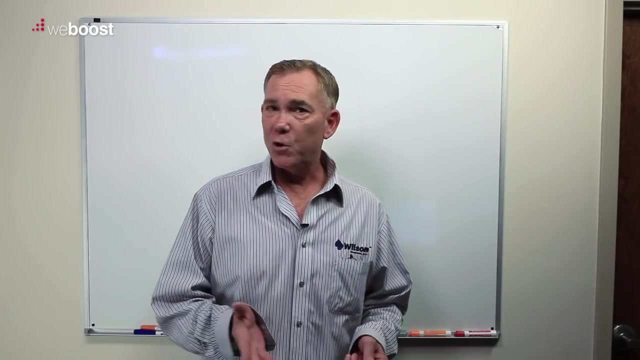 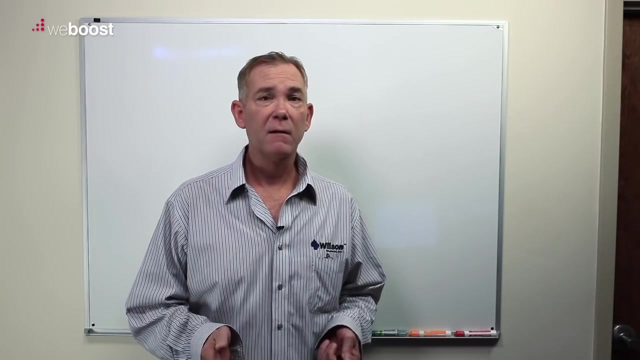 But if you notice now, the current flow is in the same direction across this plane And that allows us to generate RF energy that leaves like this and can be received as well. So if you have two pieces of wire side by side, the electromagnetic energy that is generated from current flow. 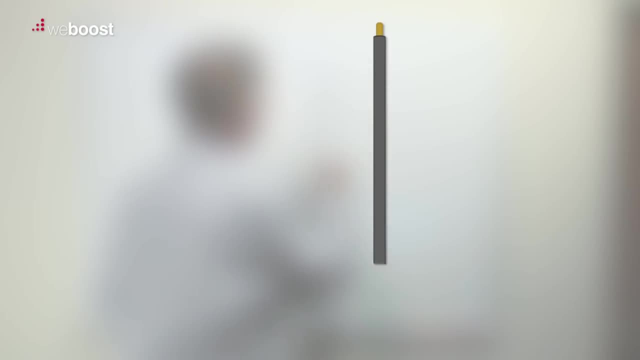 cancel each other out. So if I have a wire here and I have a wire here, this one we'll call it positive and this one we'll call negative, Because this one's positive and this one's negative, you can't get any energy to radiate out, because they cancel each other. 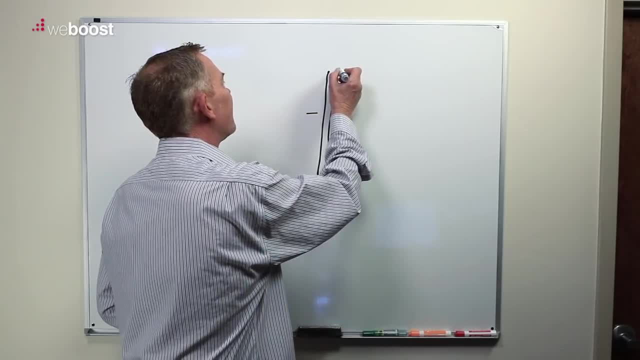 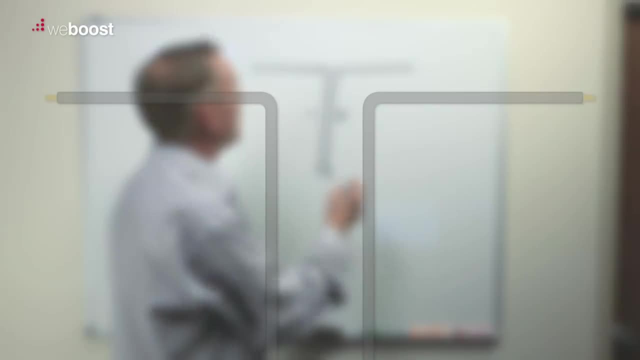 out. I think that's pretty simple. But if I take and I separate these two wires like this, so this is still my feed point down here and I have current flow in this direction and in this direction, and I have current flow in this direction and in this direction. 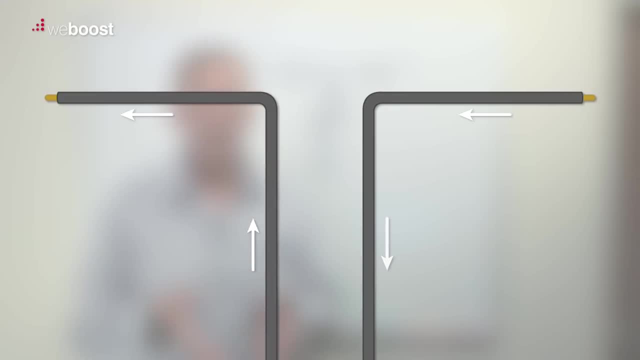 But every time you have current flow, you also have electromagnetic energy. So now, because I have current flow in the same direction across this plane, now I have an energy field that looks like this: I have a high current point here and a low current. 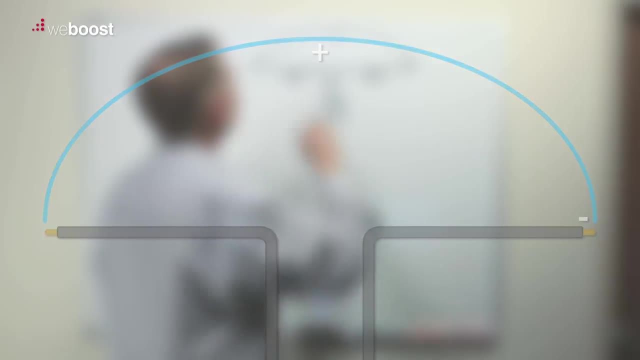 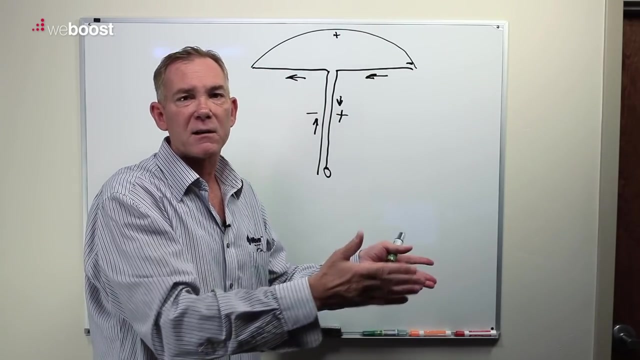 point here, but a high voltage point here, And when that high voltage point hits there, all that electromagnetic energy jumps off the wire and radiates out into space. That's basically how an antenna works. Most antennas act very similar to a dipole.